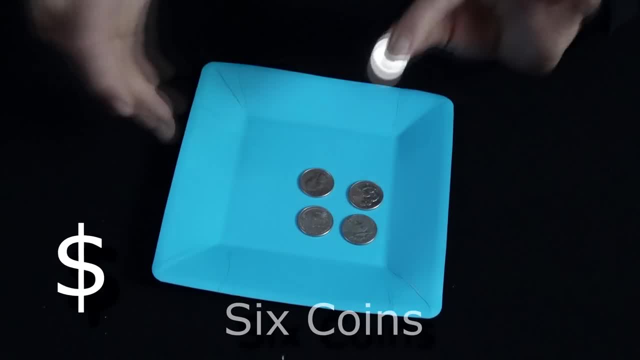 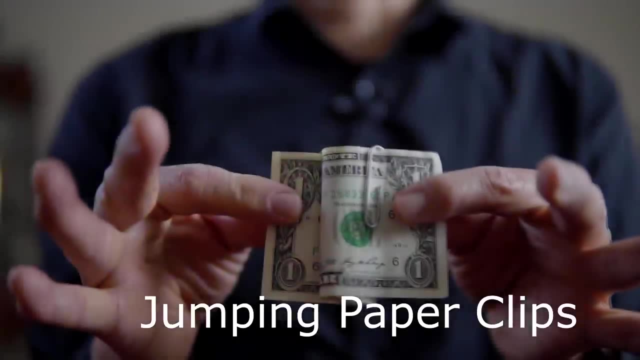 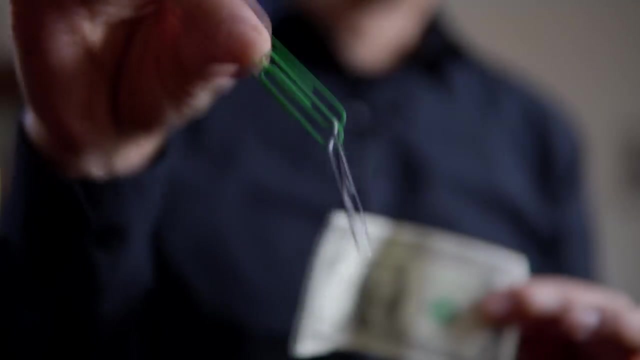 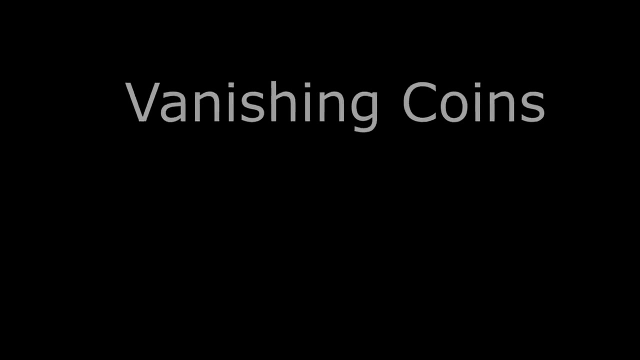 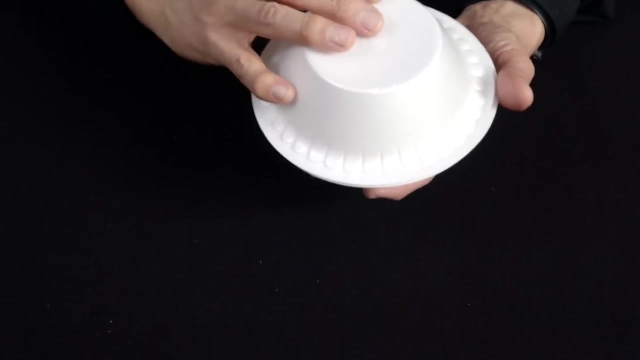 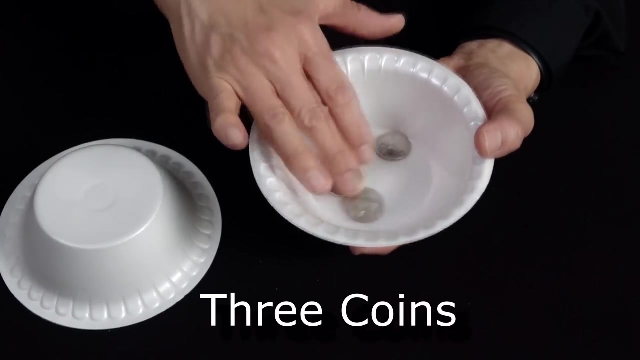 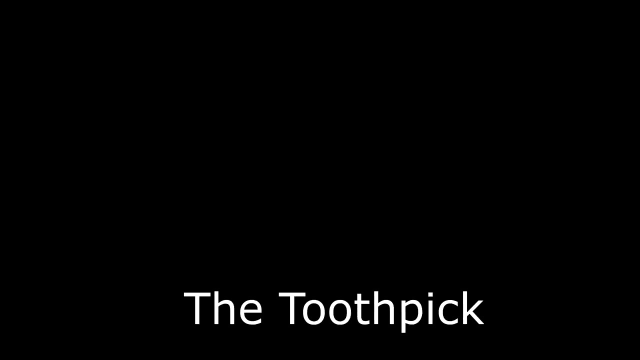 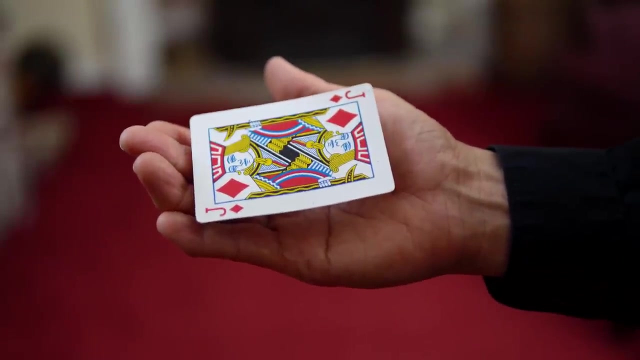 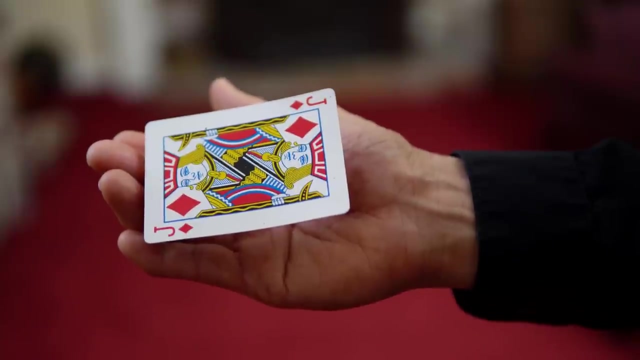 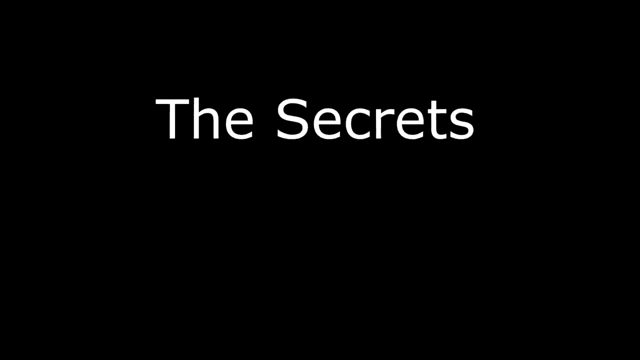 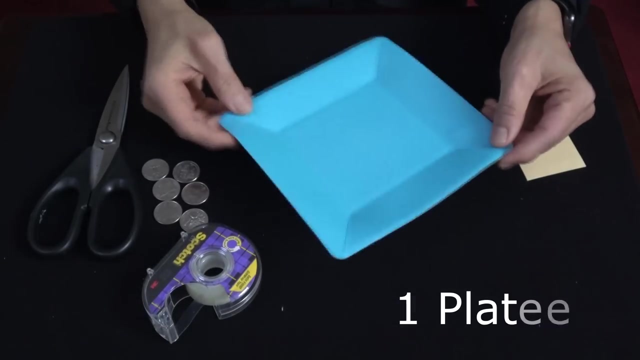 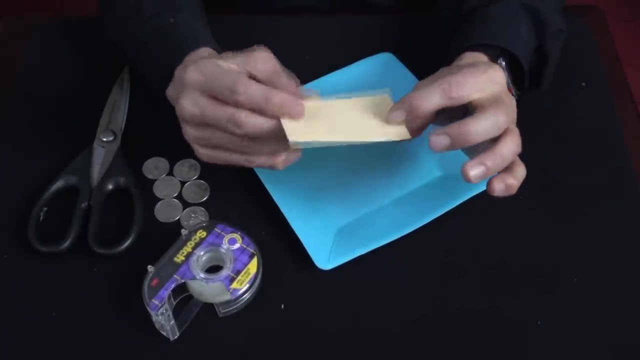 Here we go, Here we go, Here we go. For this trick you're going to need a plate. We just have a paper party plate here. I'm using an envelope, but you can actually fashion something similar out of paper, and once you see how I use the envelope, I think it'll be very 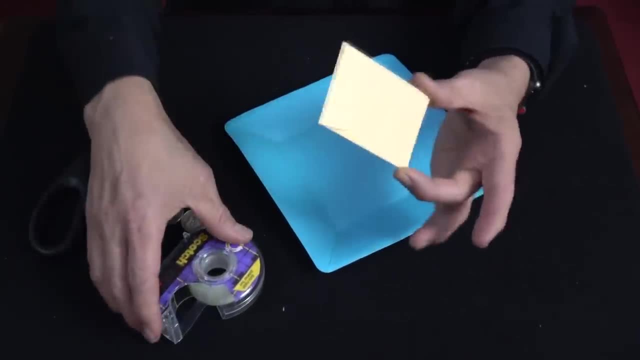 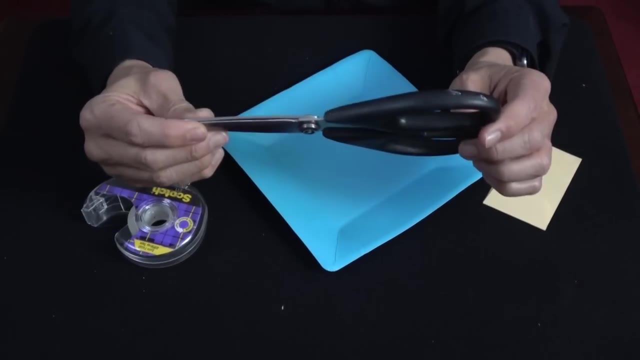 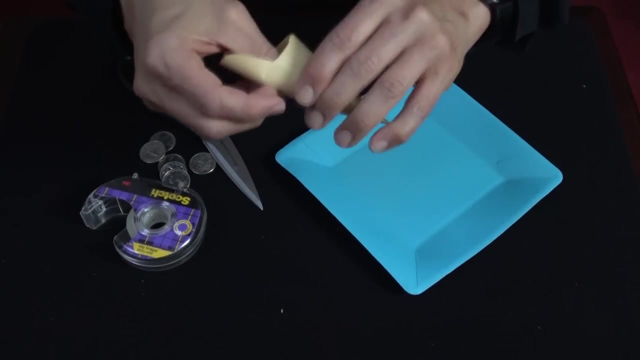 clear how you can just use some paper and some tape to make that happen, and of course you have some tape here. You're going to need some coins and, for purposes of the gimmick, you're going to need some scissors, more than likely. So I'm using a coin envelope and all I'm interested in doing I'm going to cut the 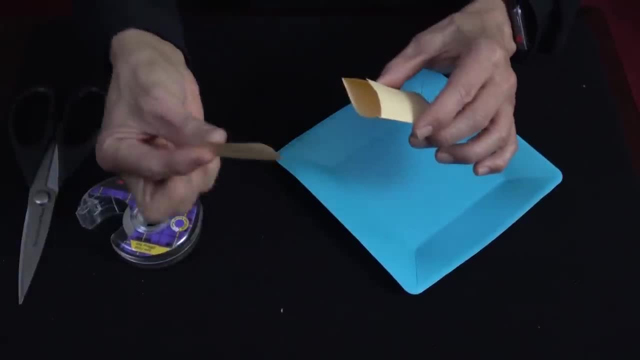 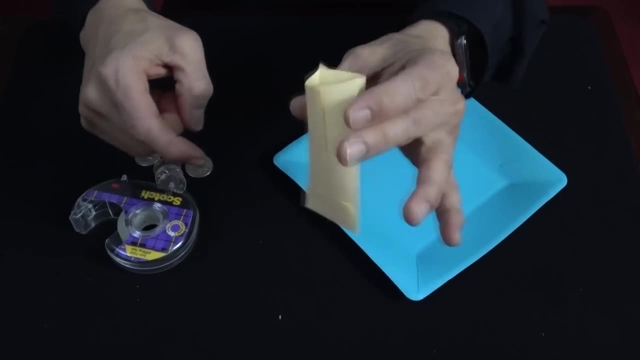 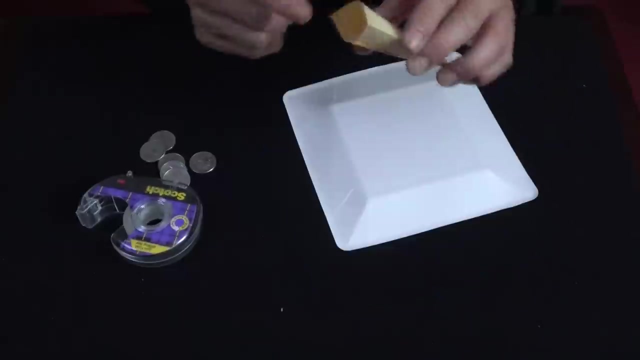 top of the flap off here. All I pretty much need is an envelope in this shape, Just enough to hold things, And you can see how you can easily fashion something like that with some paper. You take your envelope, you're going to take some tape and you're. 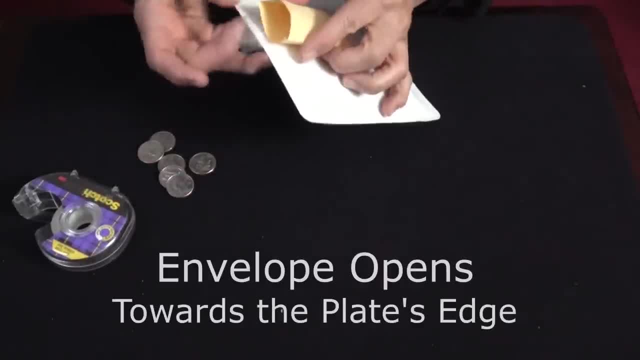 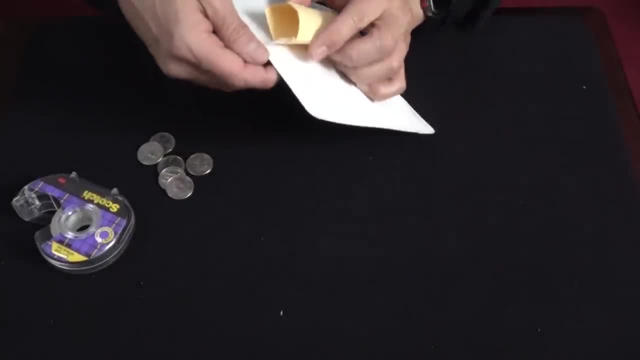 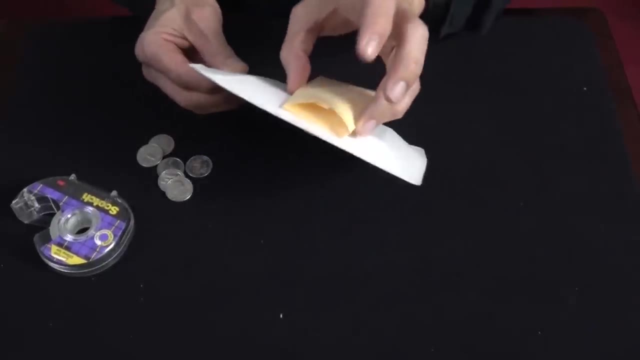 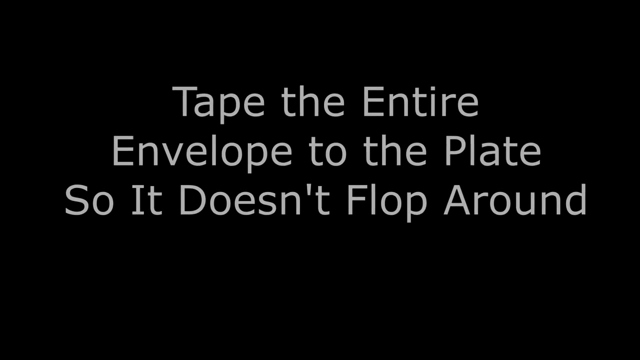 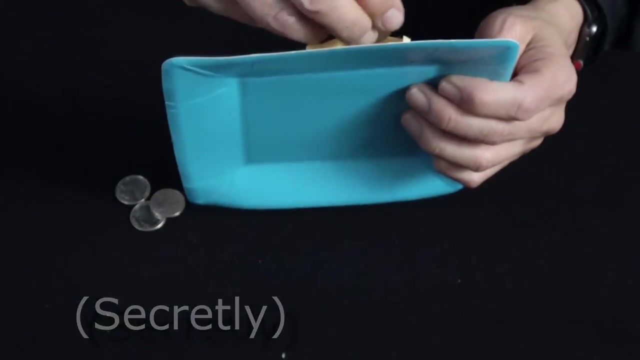 going to tape it to the edge of your plate underneath, And so you have a secret pocket Under here, which is the secret. You're ready to perform the trick. You take your three coins, load them into your secret pocket, Ready to perform the trick. You show the plate, show your hands. 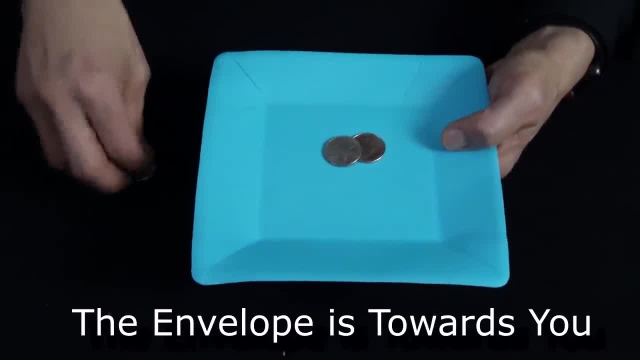 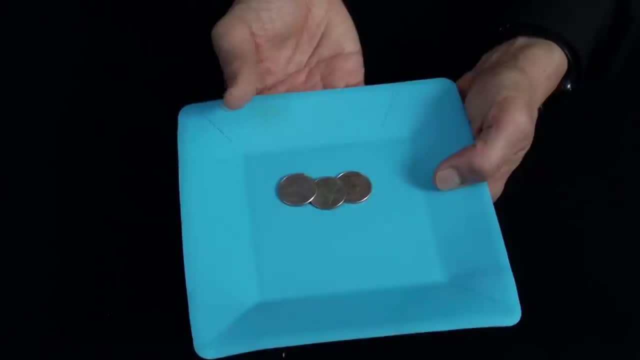 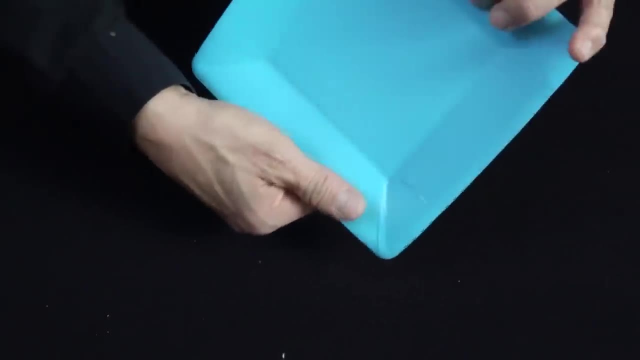 empty and you clearly count in the plate One, two, three coins. Now take your other hand, place it under the envelope here, The fingers go under the envelope and then, when you pour out all the coins, the coins from inside of the envelope come out and land in your hand. 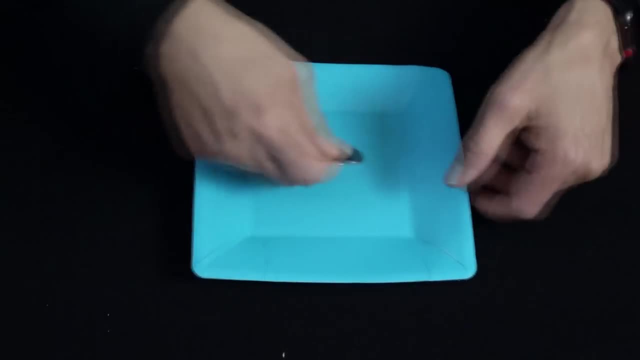 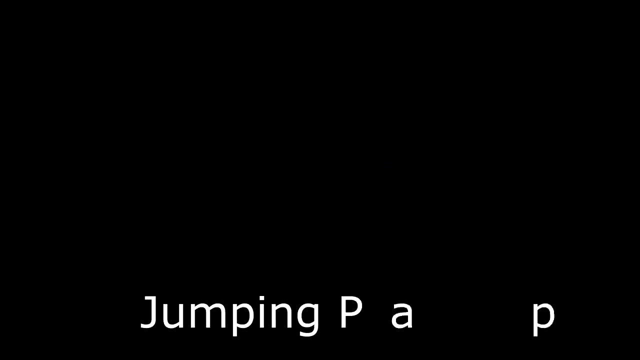 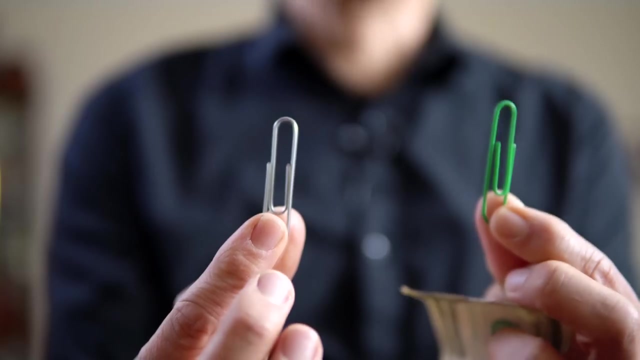 Spectators don't know this at this point. And then you can clearly count the coins: One, two, three, four, five, six coins. In this trick, you challenge spectators to link two paper clips without touching them. How can you do this? Well, here's how. 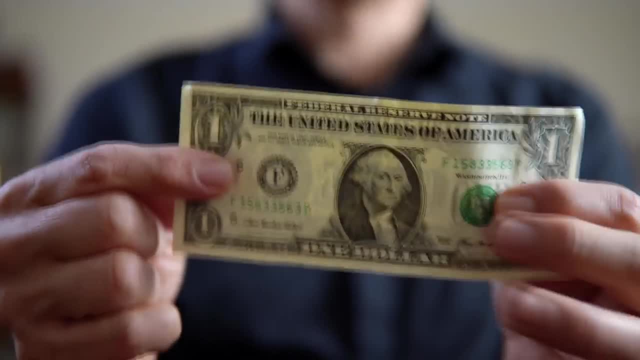 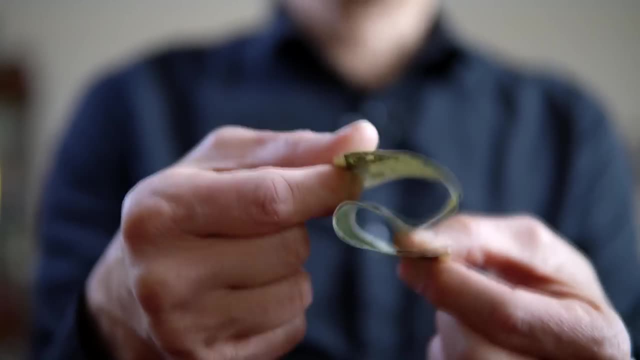 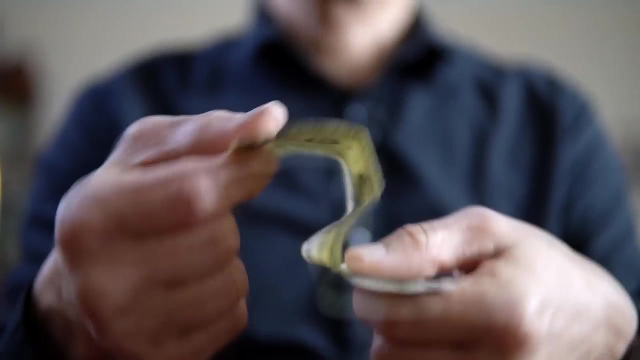 You take a dollar bill and you form it into an S. That's a reverse S to you, but it's an S to me. Okay, there's an S to you, right there, Either way, or you can call it a Z, whatever. 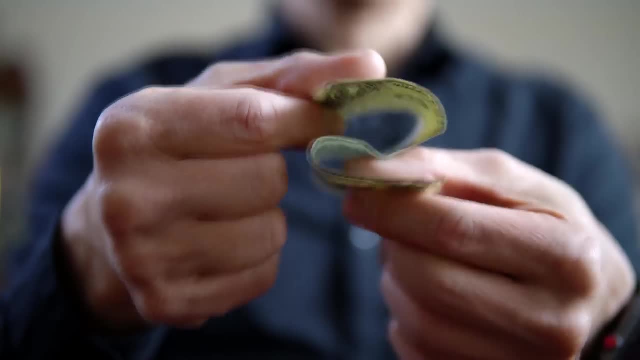 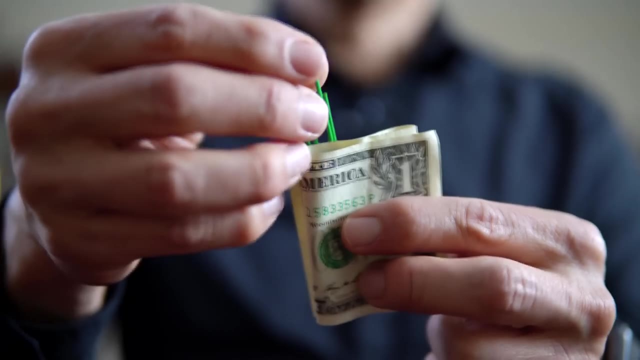 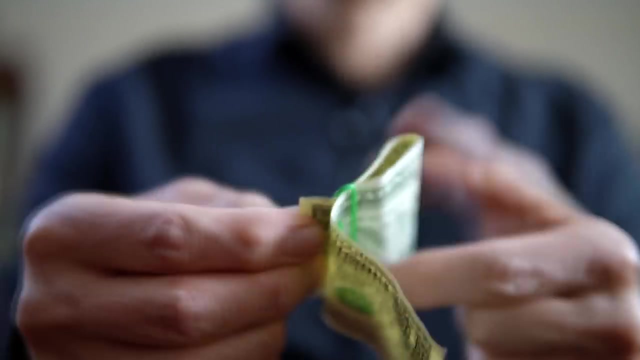 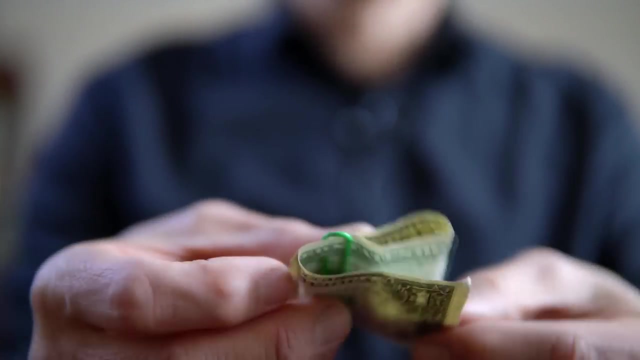 you like, You're going to just zigzag the bill like this. Now take your paper paper clips. You have two paper clips. One clip you clip right there linking this here to this here. Second of all, still form that reverse S from your perspective. Now take the second clip, place it. 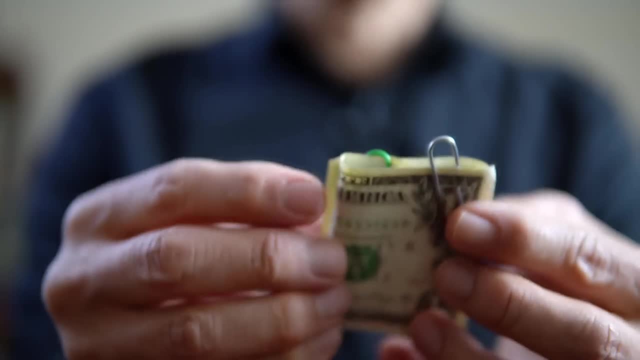 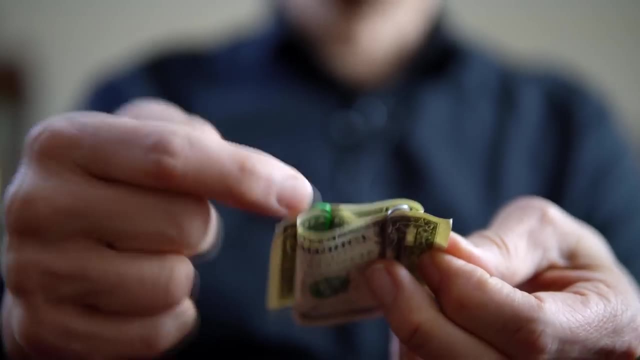 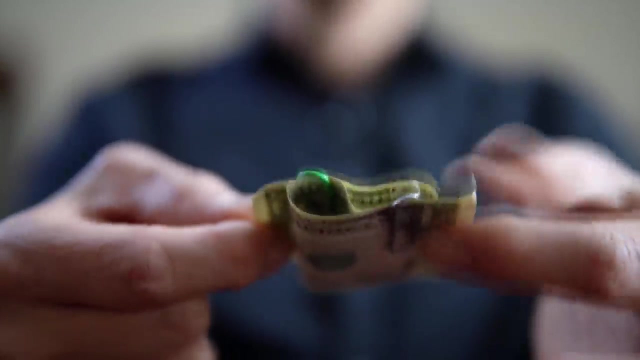 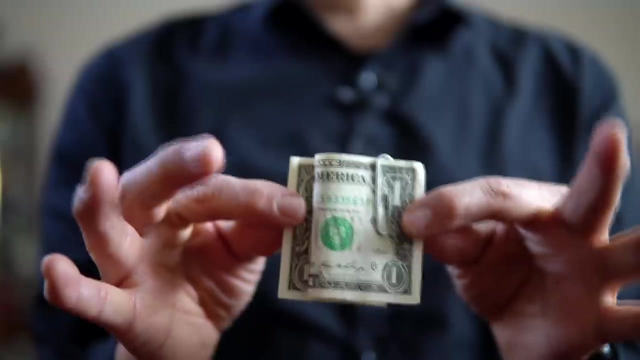 there. So you've essentially clipped the ends of the S to the centers, So now you can get a good view of it right there. Hopefully that's clear. Now the trick works itself. At this point you will not touch the paper clips, but by simply pulling these two ends the clips will magically link. 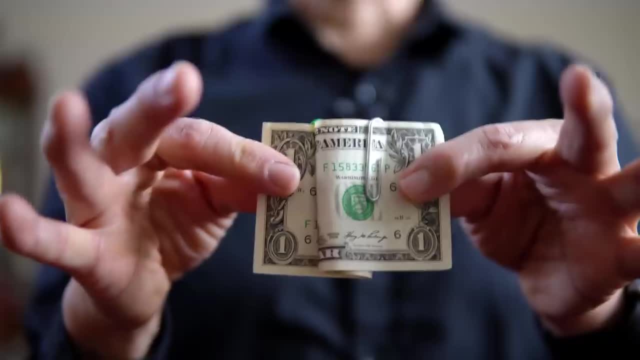 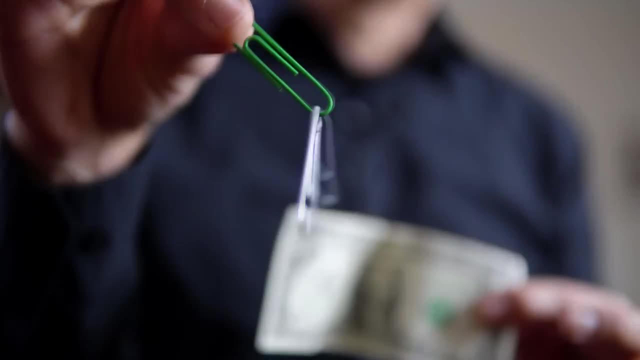 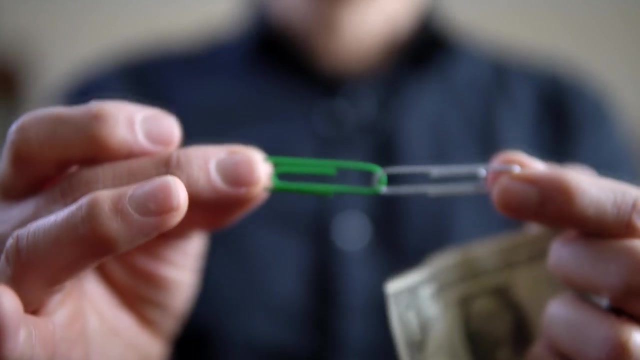 together. So now you have a good view of the S to the center. So now you can get a good view of jump off of the dollar bill. So I'm going to pull and and you'll see the paper clips are linked. perhaps it's more of a puzzle while a magic trick- cool to see these paper clips linking right in. 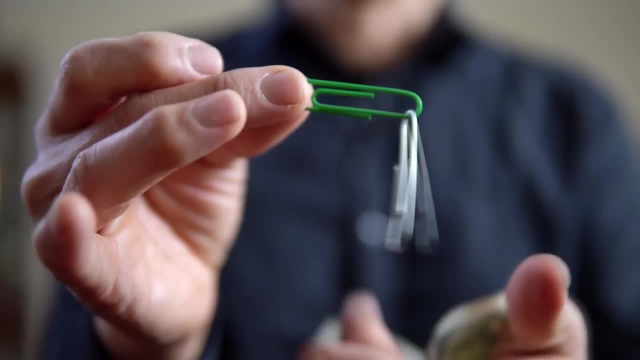 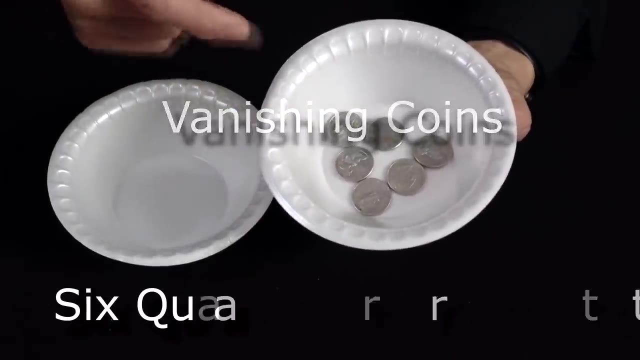 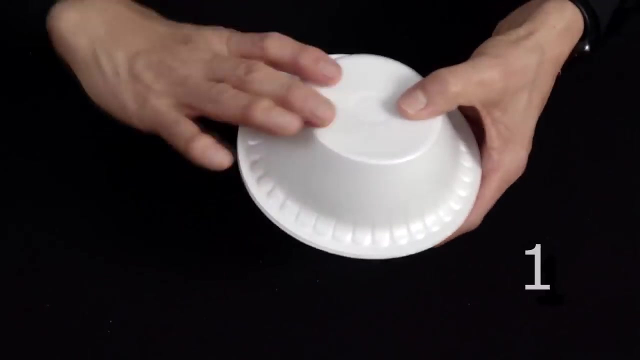 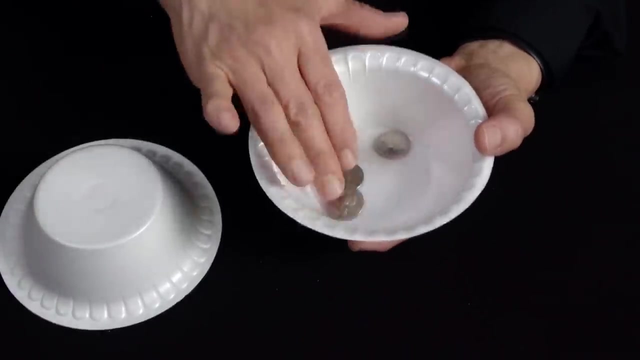 front of spectators eyes, and this is a classic magic trick for young kids. check it out. there's six quarters in here: one, two, three, four, five, six quarters. take the other bowl, place it on top. I go- one, two, three and with a snap of the finger, check it out, some money has. 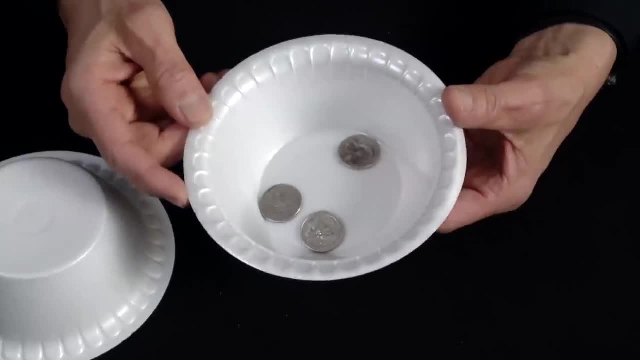 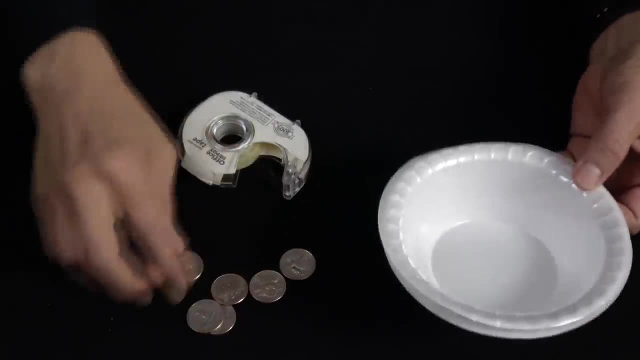 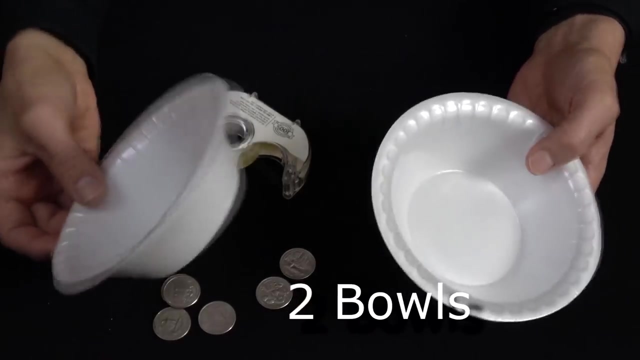 actually vanished. I don't know if anybody really needs magic to make money disappear, but just a little trick here. here's what you're gonna need for the vanishing coins. you're gonna need some quarters. I have six here. you're gonna need two bowls. these are just foam bowls. any kind of cardboard bowl will do, and 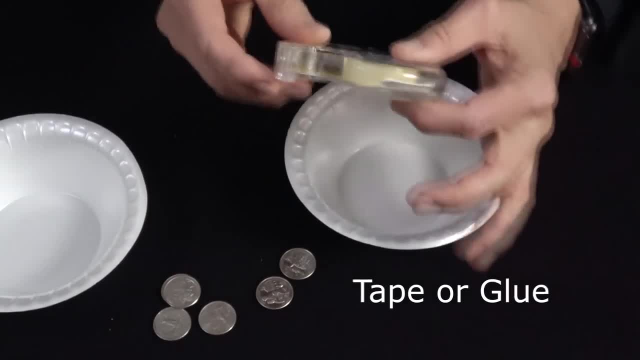 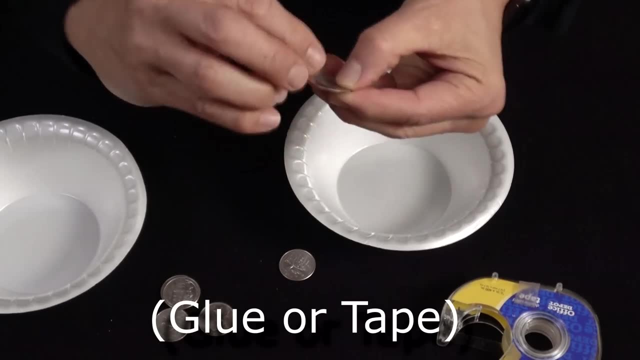 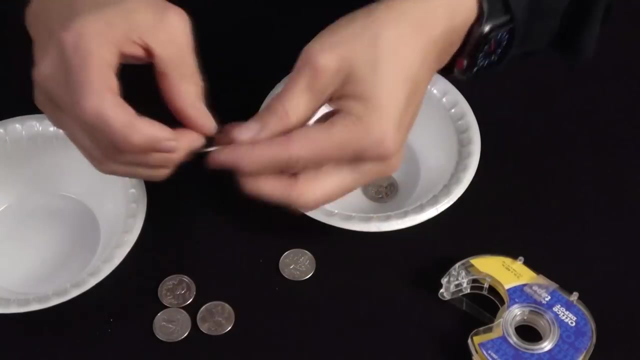 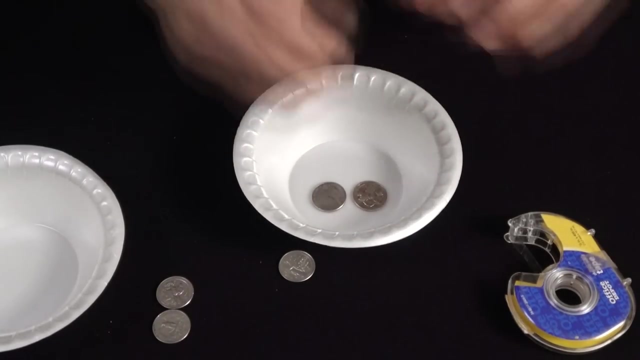 you're gonna need some glue or tape. I'm gonna use a double-sided tape here, but you can use just regular tape. all you do is take the tape and you're gonna glue three of the quarters on the bottom of one of the bowls. you now you have three quarters glued to the bottom of the bowl. they're not going. 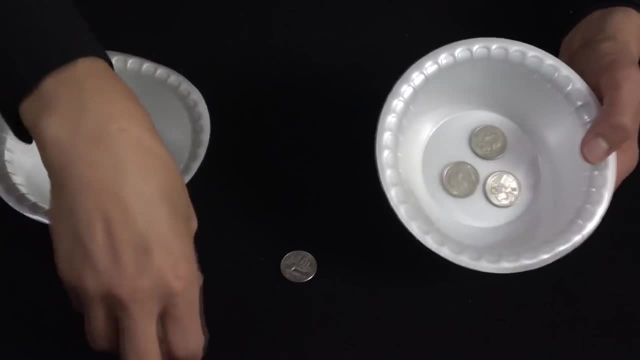 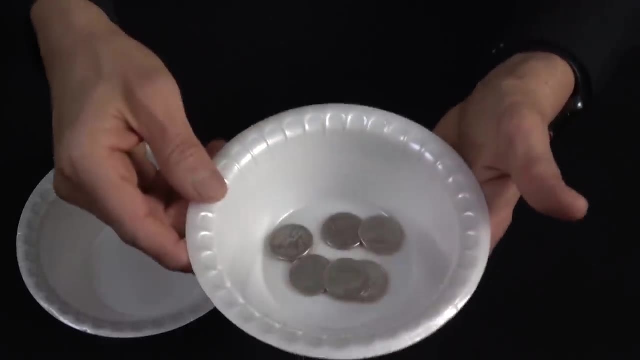 anywhere and you're ready to perform the trick. here's how. first of all, you take your other three quarters, place them in the bowl and you just walk out, show the bowl and allow spectators to count the number of quarters inside: one, two, three, four, five, six, seven, eight, nine, ten- and you're ready to go. now let's go ahead and 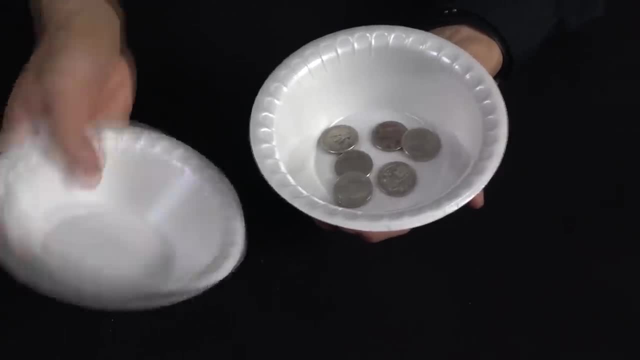 and you're ready to go now, let's go ahead. and and you're ready to go now, let's go ahead. and four five six is what they'll see. four five six is what they'll see. four five six is what they'll see. take your bowl place, the second bowl over. 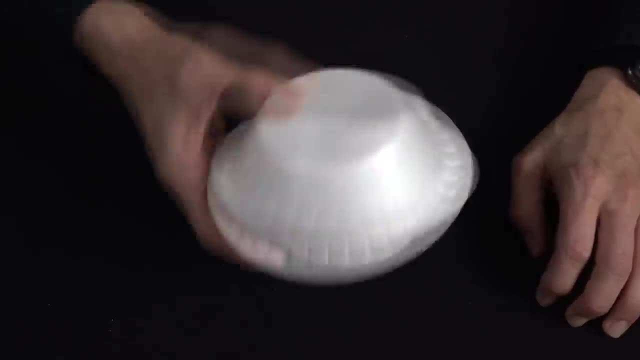 take your bowl place the second bowl over, take your bowl place the second bowl over the top, and now you're gonna turn it the top, and now you're gonna turn it the top, and now you're gonna turn it over three times. that's one, two, three. 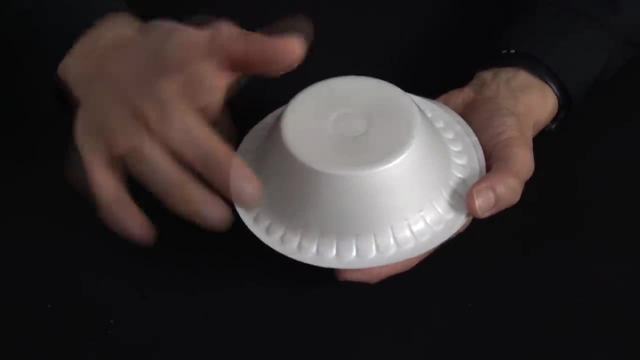 over three times. that's one, two, three over three times. that's one, two, three. remove the top of the bowl. maybe snap remove the top of the bowl. maybe snap remove the top of the bowl. maybe snap your finger for a little effect and when your finger for a little effect and when. 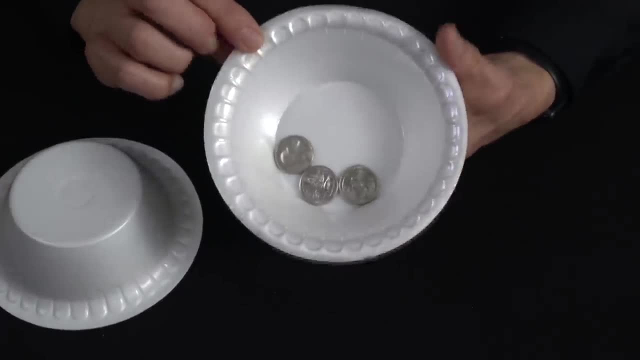 your finger for a little effect. and when you take the bowl off of the top, there's, you take the bowl off of the top. there's, you take the bowl off of the top. there's only three coins inside of the bowl. only three coins inside of the bowl. 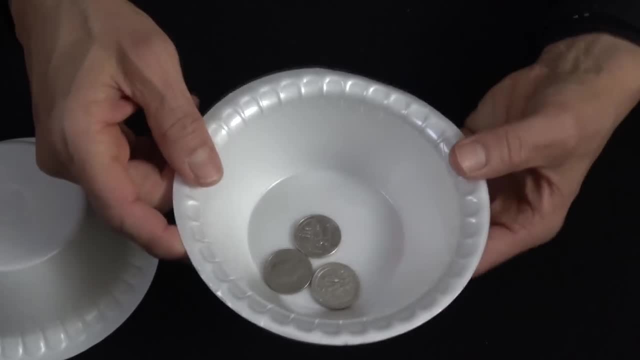 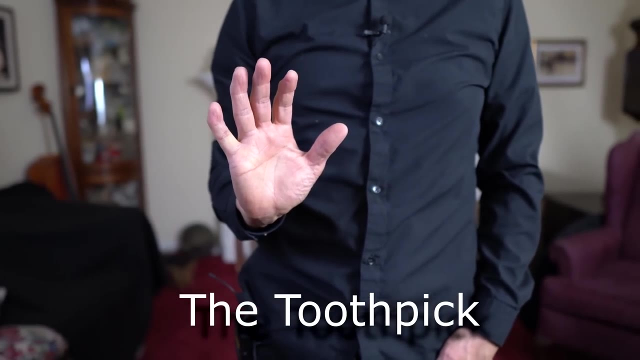 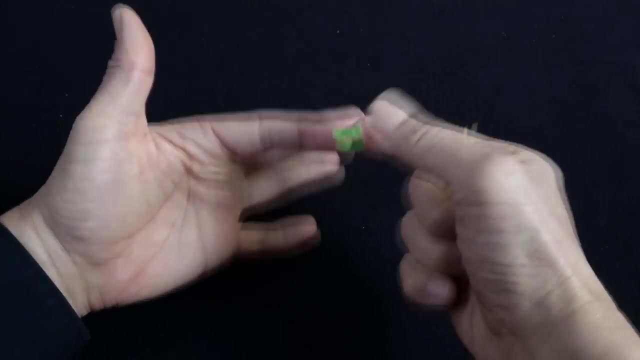 only three coins inside of the bowl. three-quarters have mysteriously- three-quarters have mysteriously- three-quarters have mysteriously vanished from your hands. what you'll need for this toothpick: what you'll need for this toothpick. what you'll need for this toothpick trick is a toothpick and a piece of tape. 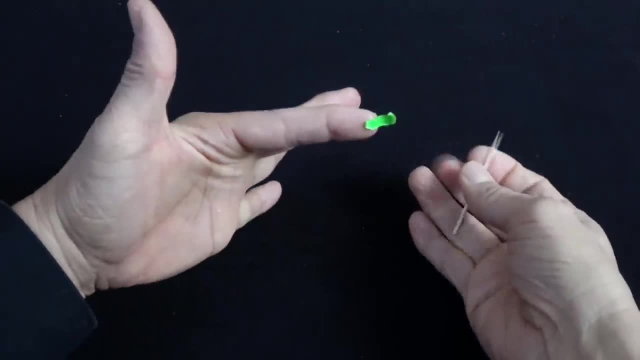 trick is a toothpick and a piece of tape. trick is a toothpick and a piece of tape. now, I would suggest you use clear tape now. I would suggest you use clear tape now. I would suggest you use clear tape. I'm using a piece of bright green tape. 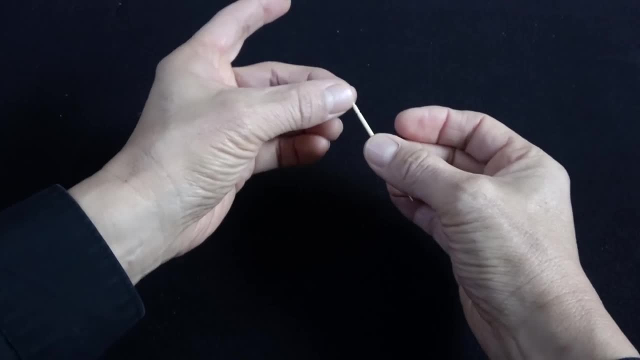 I'm using a piece of bright green tape. I'm using a piece of bright green tape here for explanation purposes. it's a lot here for explanation purposes. it's a lot here for explanation purposes. it's a lot easier, I think, for you to see now what. 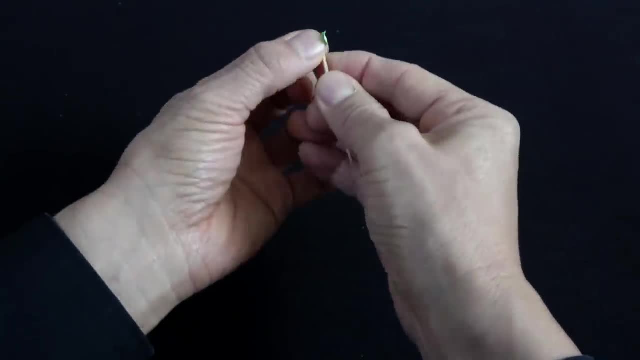 easier, I think, for you to see now what easier I think for you to see now what you do is just take your toothpick and you do is just take your toothpick and you do is just take your toothpick and put the little piece of tape on it and 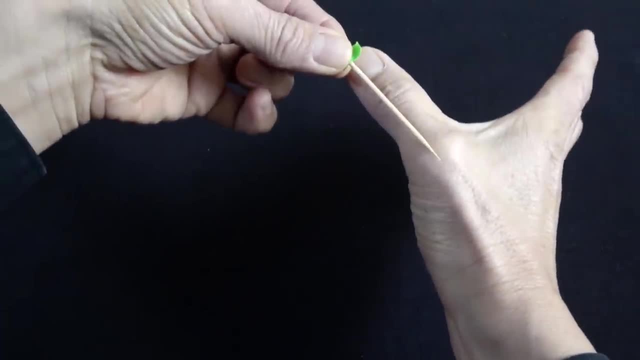 put the little piece of tape on it and put the little piece of tape on it and now you're going to tape it onto your. now you're going to tape it onto your. now you're going to tape it onto your back of your thumbnail once you have it. 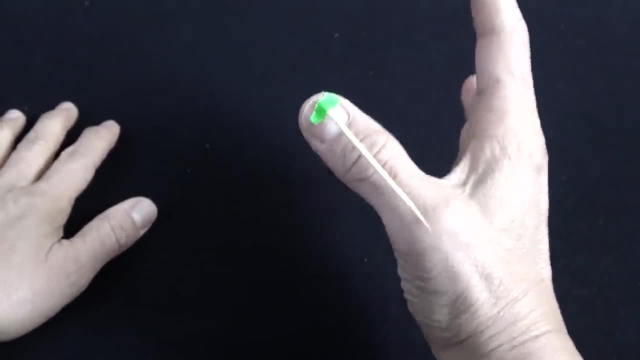 back of your thumbnail. once you have it back of your thumbnail, once you have it taped to your thumb, you're ready to taped to your thumb. you're ready to taped to your thumb. you're ready to perform the trick now. what you do is you perform the trick now. what you do is you. 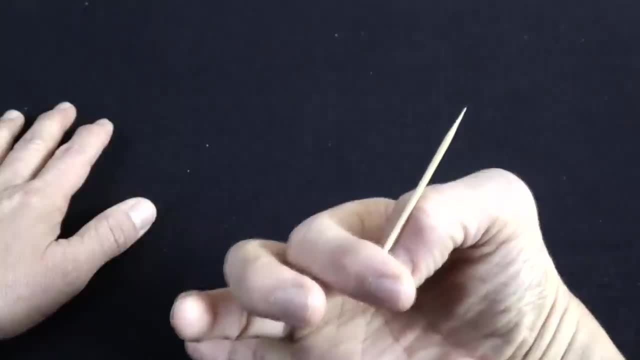 perform the trick now. what you do is you bend your thumb and hide the tape with: bend your thumb and hide the tape with. bend your thumb and hide the tape with your finger, so people see your hand and your finger. so people see your hand and your finger. so people see your hand and it looks fairly natural as if you are. 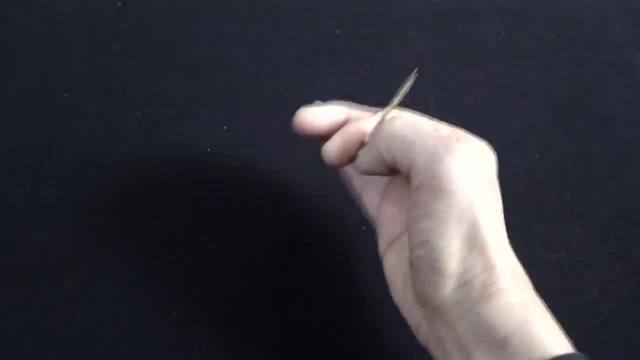 it looks fairly natural, as if you are. it looks fairly natural as if you are holding a toothpick in your fingers and holding a toothpick in your fingers and holding a toothpick in your fingers and then to make the vanish happen. you then to make the vanish happen. you. 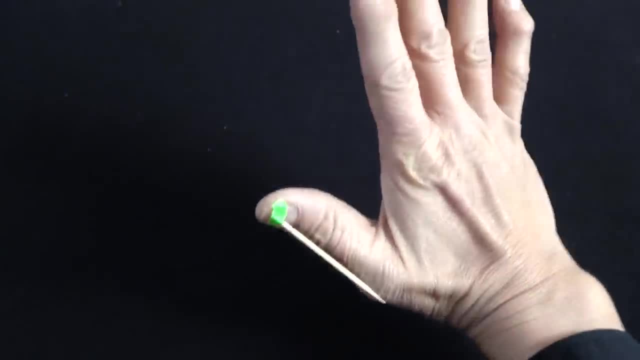 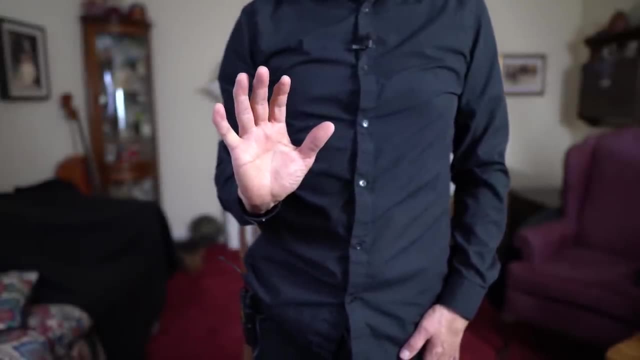 then, to make the vanish happen, you simply reach forward, flip it out, and you simply reach forward, flip it out, and you simply reach forward, flip it out and you can show your hand pretty much empty, can show your hand pretty much empty, can show your hand pretty much empty, except you have the thumb with the 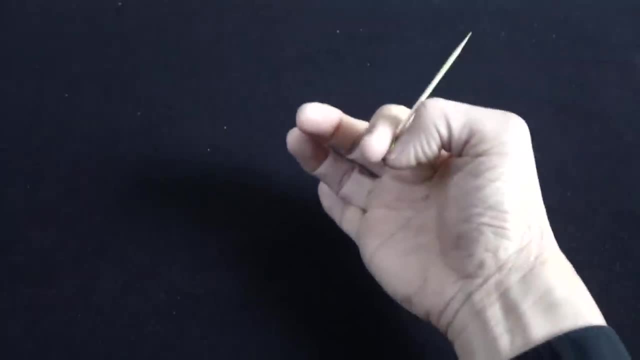 except you have the thumb with the. except you have the thumb with the toothpick behind your hand, hold it and toothpick behind your hand, hold it and toothpick behind your hand. hold it and it vanishes in your hand. just make sure it vanishes in your hand, just make sure. 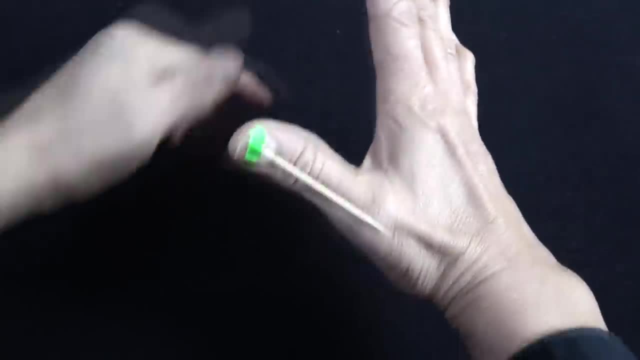 it vanishes in your hand. just make sure that the line of sight of your, that the line of sight of your, that the line of sight of your spectators is looking this way and that spectators is looking this way and that spectators is looking this way, and that the toothpick is hidden if you start to. 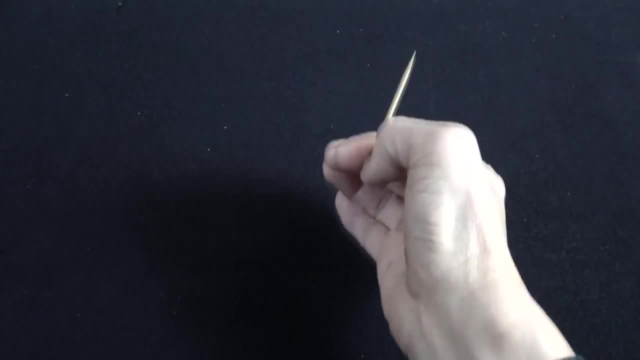 the toothpick is hidden. if you start to, the toothpick is hidden. if you start to turn, obviously they will see the turn, obviously they will see the turn, obviously they will see the toothpick and that is the toothpick trick, toothpick and that is the toothpick trick. 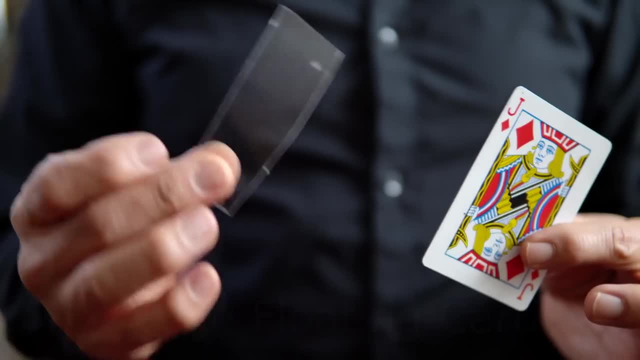 toothpick, and that is the toothpick trick. what you'll need for this trick is a. what you'll need for this trick is a. what you'll need for this trick is a playing card and a piece of flexible playing card and a piece of flexible playing card and a piece of flexible plastic you can get this off of in. 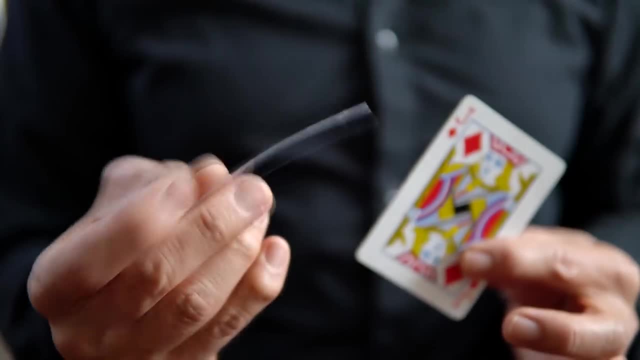 plastic. you can get this off of in plastic. you can get this off of in almost any kind of packaging. you can almost any kind of packaging. you can almost any kind of packaging. you can have a salad mixed. they're everywhere. have a salad mixed, they're everywhere. 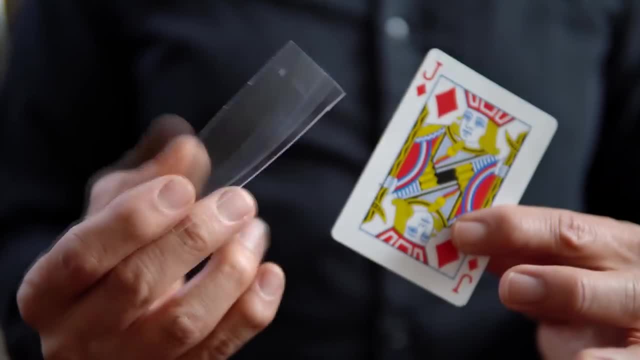 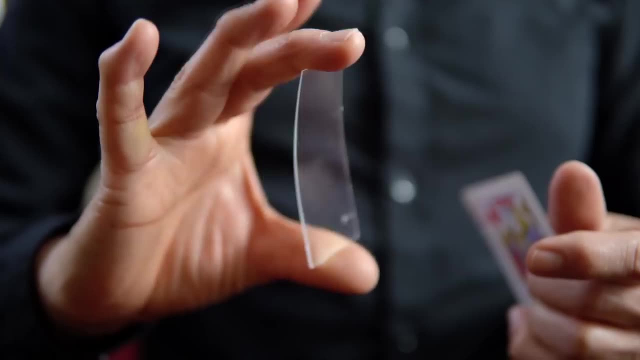 have a salad mixed. they're everywhere in cups that you get at the, the coffee in cups that you get at the, the coffee in cups that you get at the, the coffee shop. just find a piece of flexible shop. just find a piece of flexible shop, just find a piece of flexible plastic. and that's the secret to the. 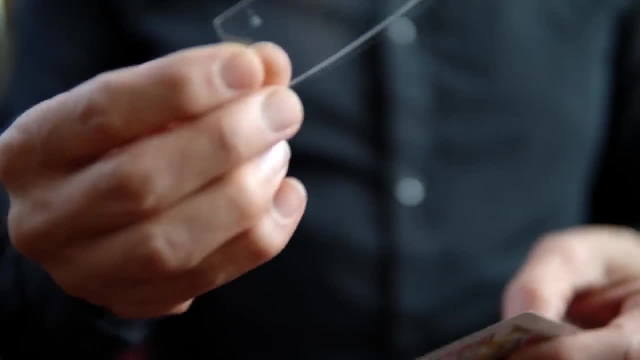 plastic and that's the secret to the plastic and that's the secret to the trick. and you're gonna need some tape trick and you're gonna need some tape trick and you're gonna need some tape. so cut this piece of plastic. maybe about. so cut this piece of plastic, maybe about. 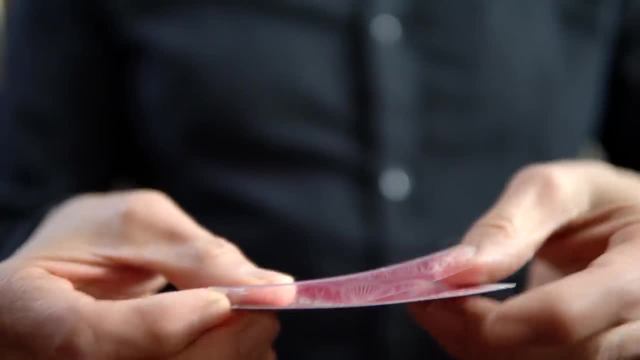 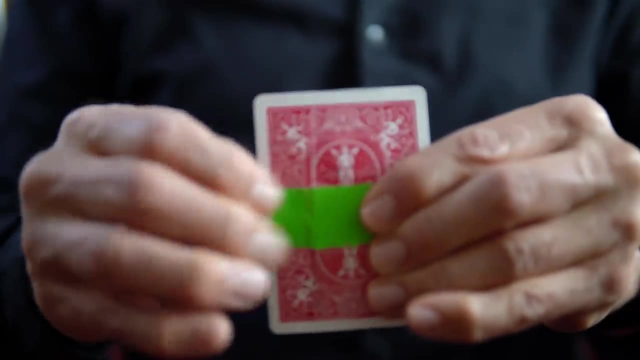 so cut this piece of plastic, maybe about an inch here, and then the length would an inch here, and then the length would an inch here, and then the length would be the same length as a playing card. be the same length as a playing card. be the same length as a playing card here. get a couple pieces of tape or just. 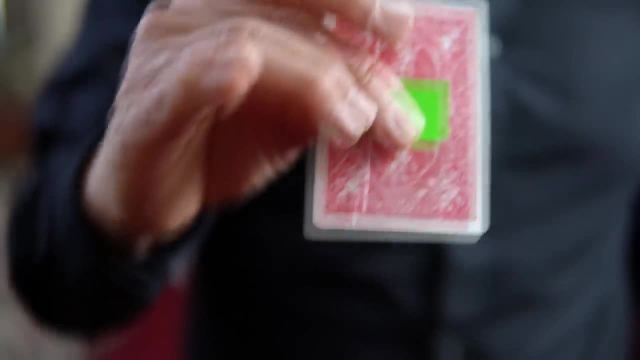 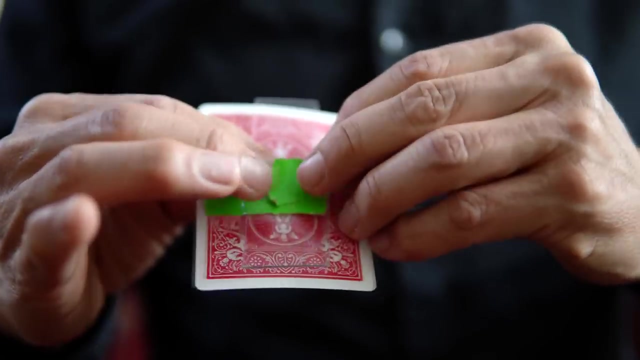 here, get a couple pieces of tape. or just here, get a couple pieces of tape, or just one tape: the piece of plastic to the one tape, the piece of plastic to the one tape, the piece of plastic to the back of the card. now I'm using green. back of the card. now I'm using green back of the card. now I'm using green tape here, so it's easier to tape here. so it's easier to tape here, so it's easier to for me to demonstrate what this looks, for me to demonstrate what this looks. 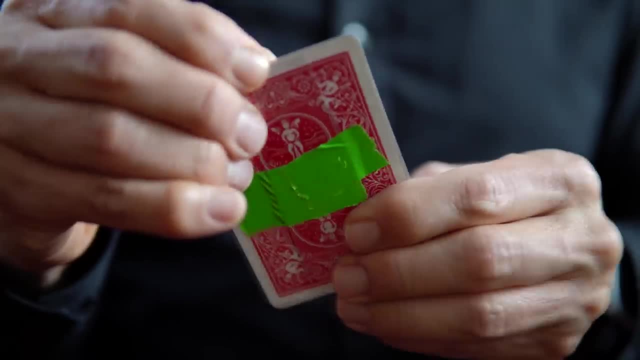 for me to demonstrate what this looks like. you'll probably just want to use like. you'll probably just want to use like. you'll probably just want to use clear tape. it'll work just fine. and now clear tape. it'll work just fine. and now clear tape. it'll work just fine. and now you have a piece of plastic on the back. 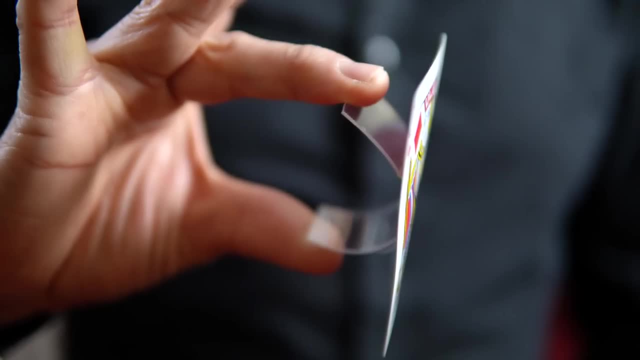 you have a piece of plastic on the back. you have a piece of plastic on the back of a playing card and when you flex the of a playing card and when you flex the of a playing card and when you flex the plastic, it bows out and causes the card. 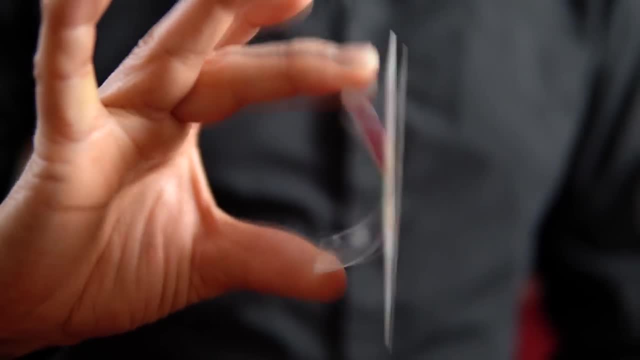 plastic. it bows out and causes the card plastic. it bows out and causes the card to seemingly rise. and that's the secret: to seemingly rise. and that's the secret to seemingly rise. and that's the secret of the trick. of the trick, I like to take the card and place it in. 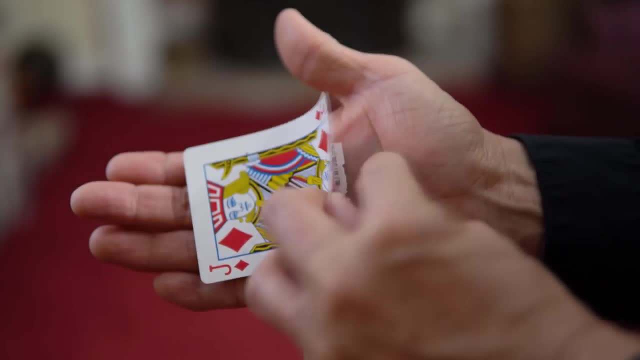 I like to take the card and place it in. I like to take the card and place it in my hand. I like to take one piece of my hand. I like to take one piece of my hand. I like to take one piece of plastic. have it along the base of the.